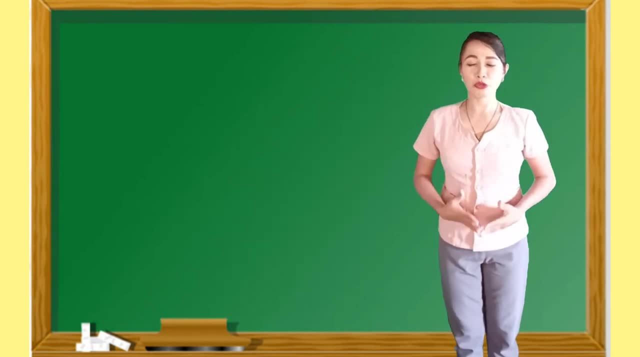 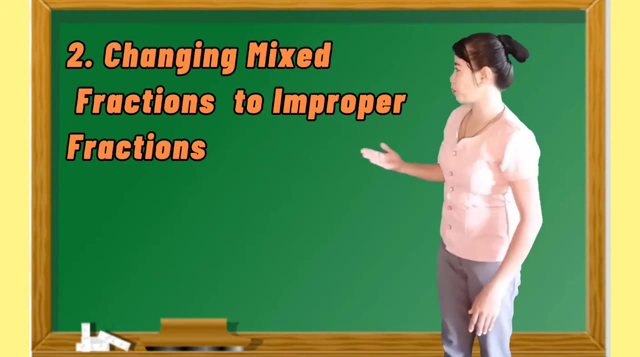 Alright. another thing that we need to review is that changing mixed fraction to improper fractions. For example, we have 2 and 3. fifth, So we have to multiply first the denominator, which is 5, and the whole number, which is 2.. 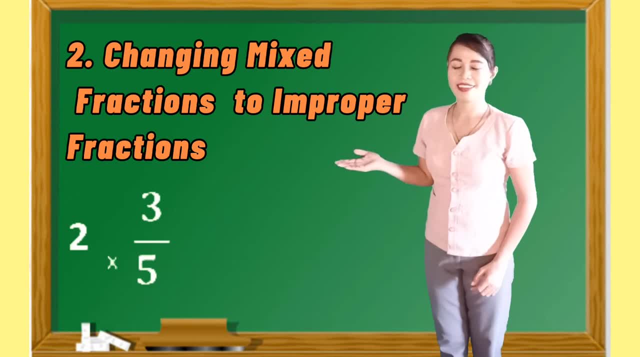 So 5 times 2 is equals to 10.. And then we are going to add the numerator, which is 3.. So 10 plus 3 is equals to 30. So 10 plus 3 is equals to 30.. 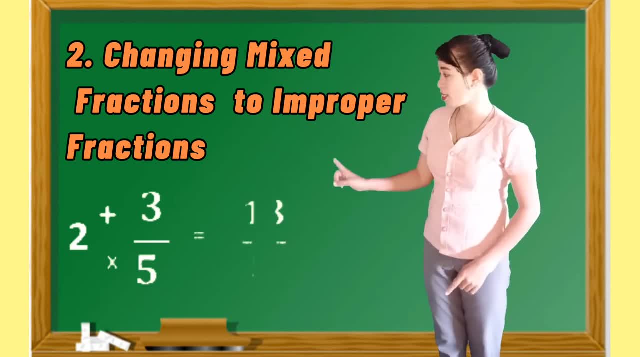 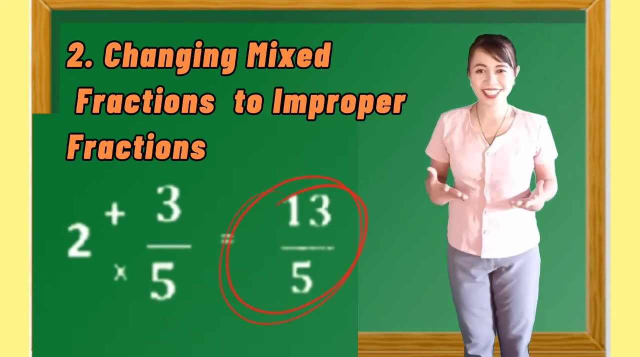 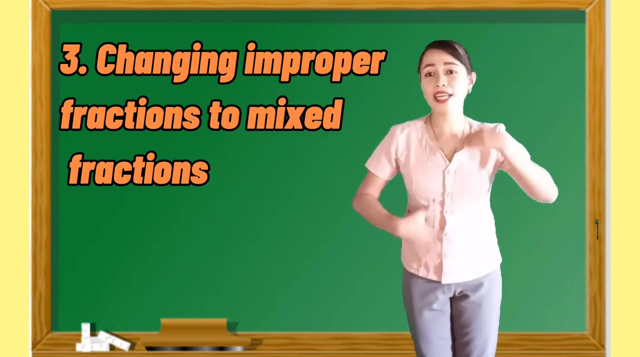 And copy only the denominator, which is 5.. So we have 13 over 5 or 13 fifth. As easy as that. And if we reverse it, changing improper fraction to mixed fraction. So let us also invert the operation. 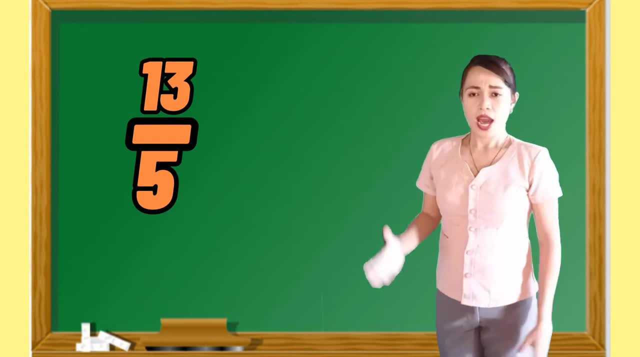 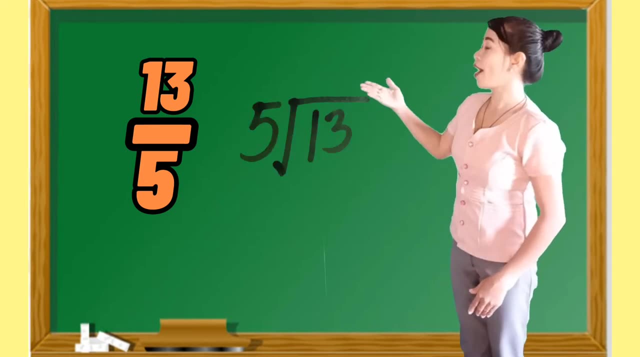 For example, we have 13. fifth, How can we do this? Alright, we have to divide 3 by 5.. We have to divide 13 as the dividend and 5 as the divisor. So we have: 13 divided by 5 is 2.. 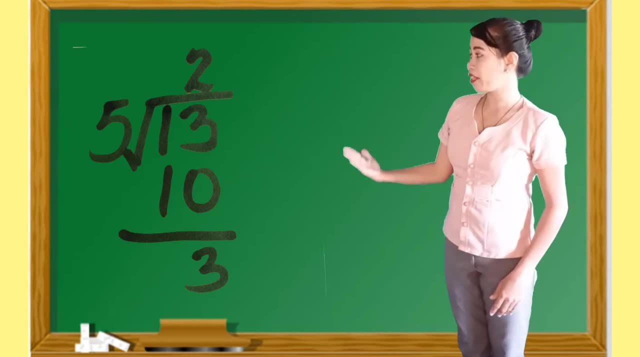 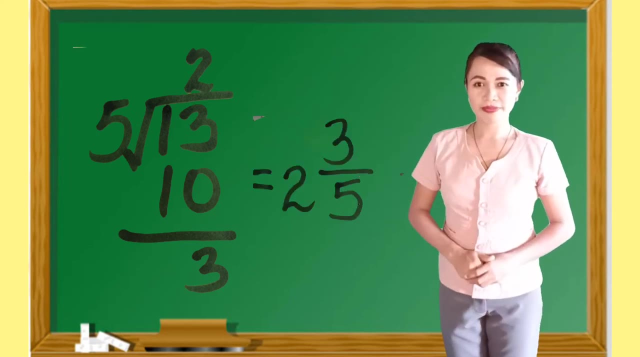 And 2 times 5 is 10.. Remainder 3.. The answer will be the whole number. The remainder, 3 is the numerator And the divisor 5 is the denominator. So 13 fifth is equals to 2 and 3 fifth. 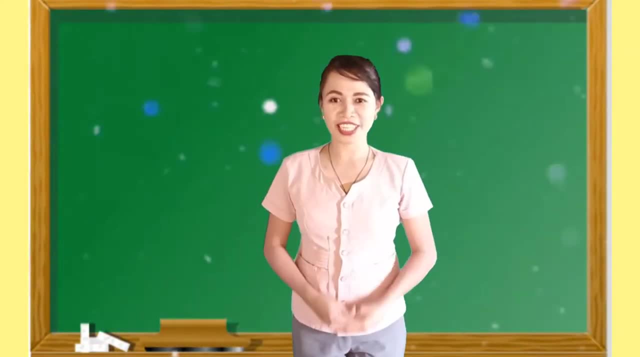 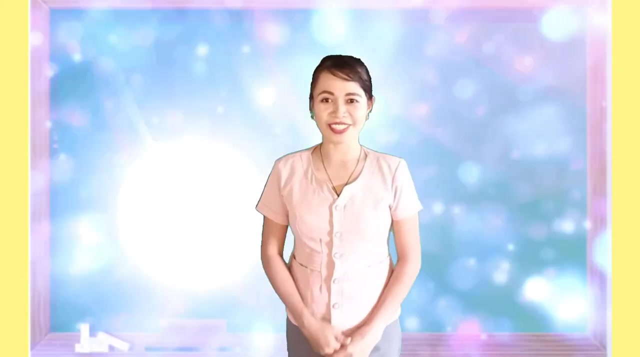 So please replay if you did not understand it yet. What do we mean? or how do we change improper fraction to mixed numbers and vice versa? Now we already done with all the necessary skills in this topic, So welcome to our new lesson. 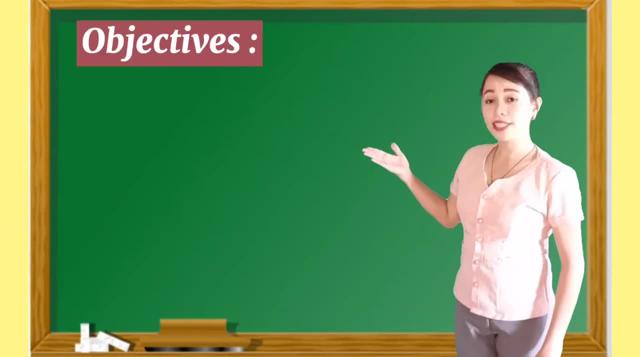 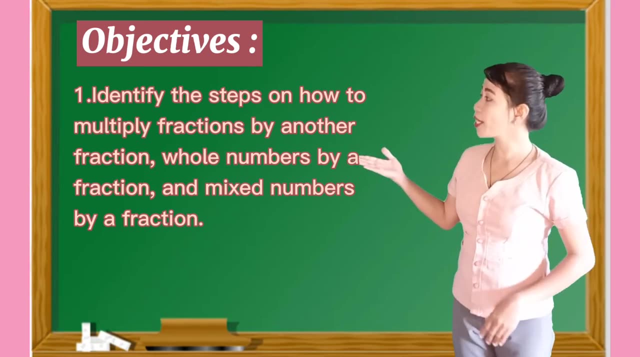 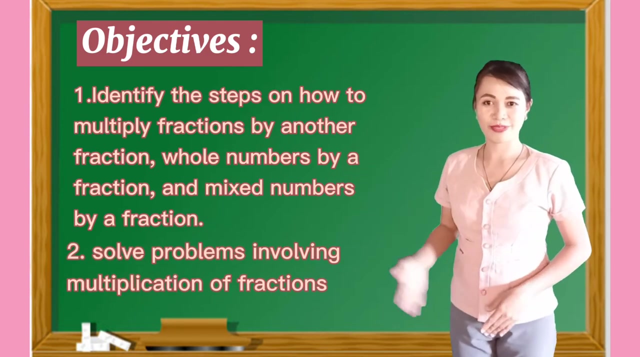 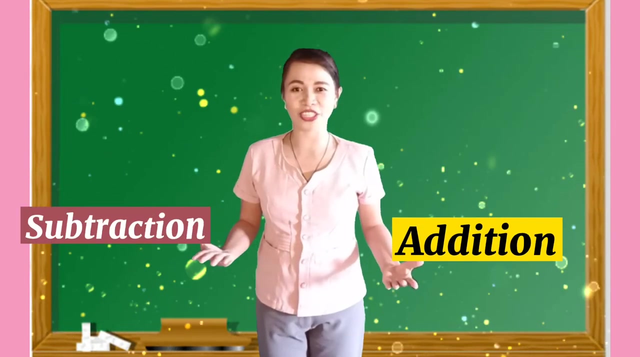 For today's lesson, you will be able to identify the steps on how to multiply another fraction. First, pull numbers by a fraction and mix numbers by a fraction. Second, solve problems involving multiplication of fractions. For this operation, I am sure that you will find this much easier than addition and subtraction. 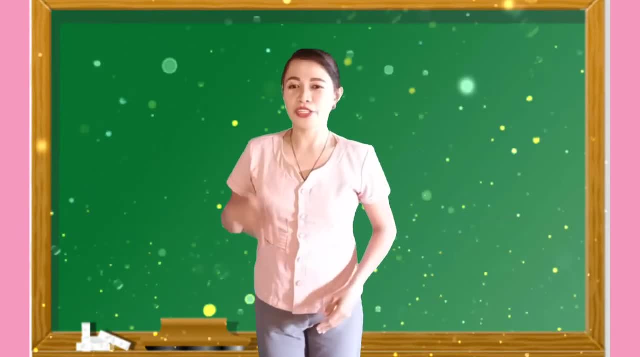 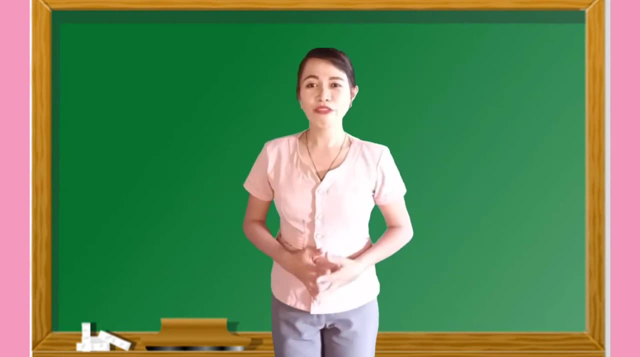 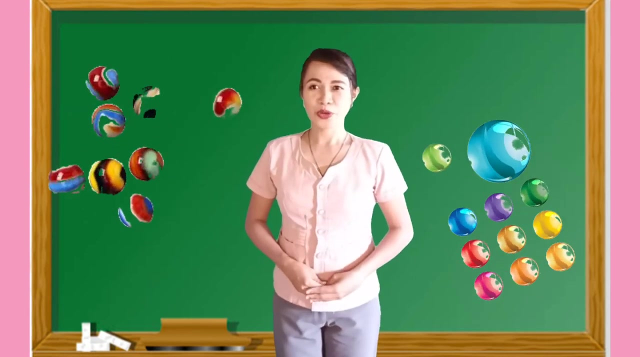 You know why? Because there's no such complicated steps here than you did in the first two operations. So now I have a question: How many of you like to play marbles? If you love marbles, will you share it to your friends? 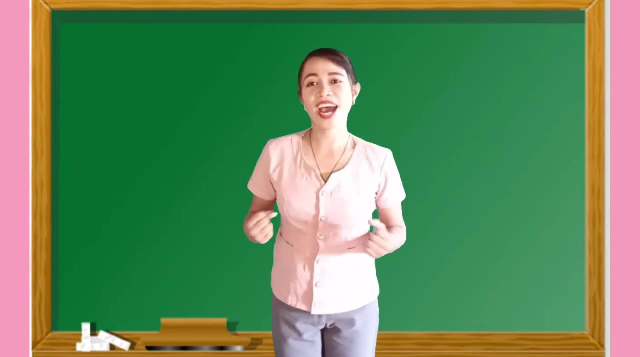 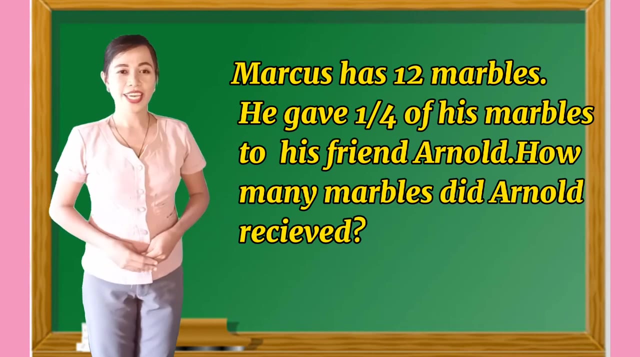 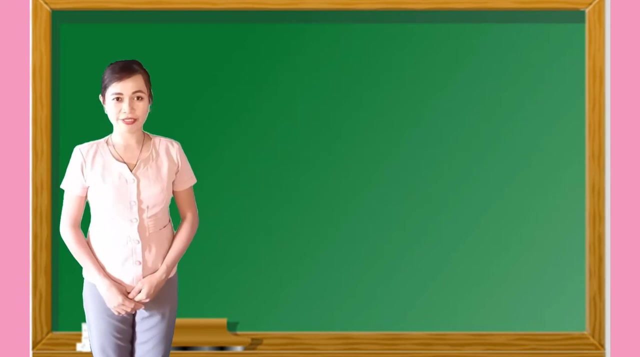 Alright, very good. So now here is the problem. Marcus has 12 marbles. He gave 1 fourth of his marbles to his friend Arnold. How many marbles did Arnold receive? So, in order for us to answer the word problem, 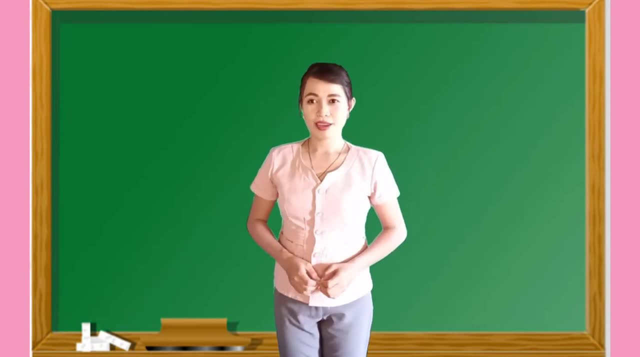 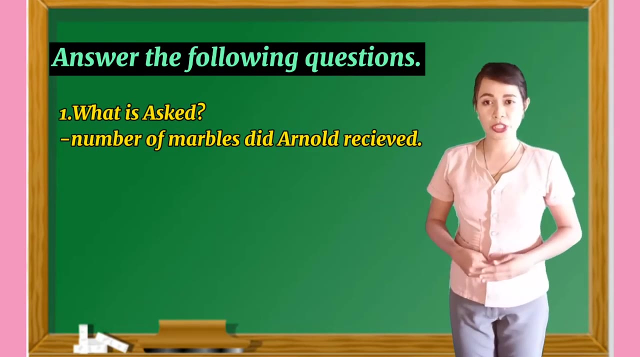 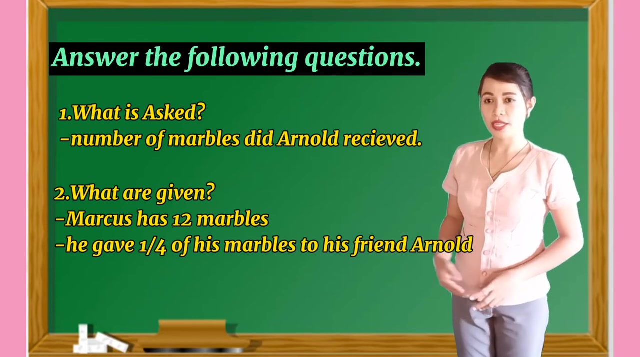 we have to answer the following guide question, Number 1. What is asked? It is the number of marbles. did Arnold receive? Number 2. What are given? Marcus has 12 marbles and he gave 1 fourth of his marbles to his friend Arnold. 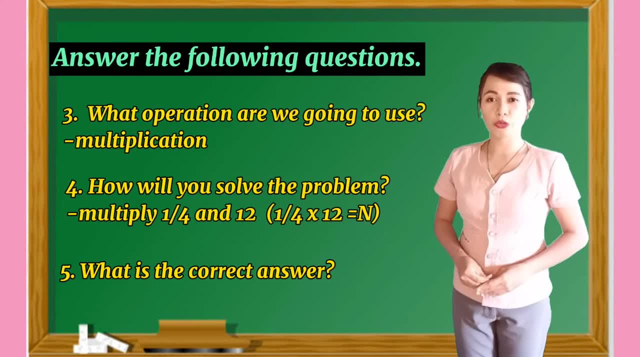 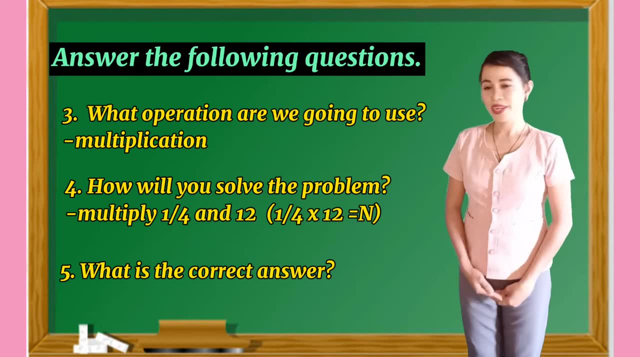 Third, what operation are we going to use? Of course, multiplication Number 4.. How will you solve the problem? By multiplying 1, fourth and 12.. Or 1 fourth times 12 is equal to n. And the last guide question is: 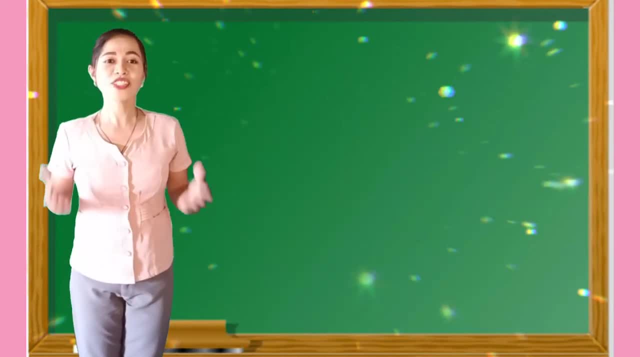 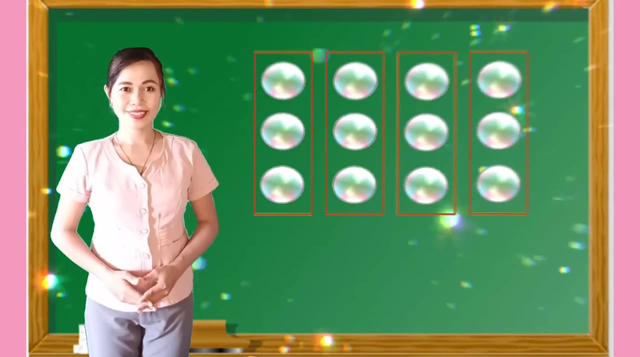 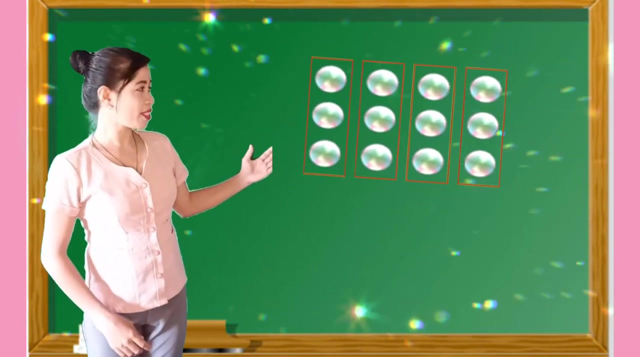 What is the correct answer To answer the problem, let us draw first a figure to represent the 1 fourth of 12 marbles. Marcus divides his marbles into 4.. Each group represents 1 fourth of his 12 marbles. 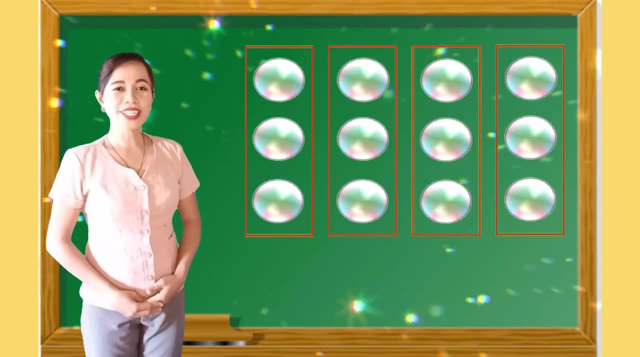 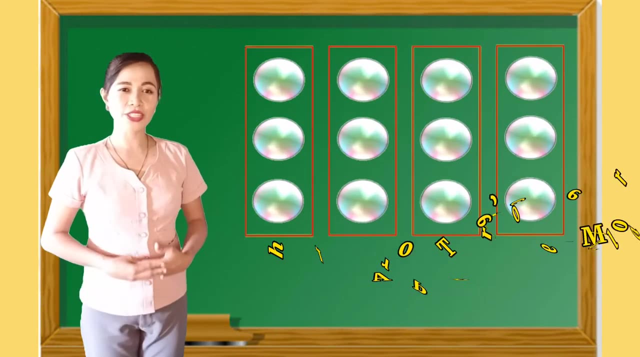 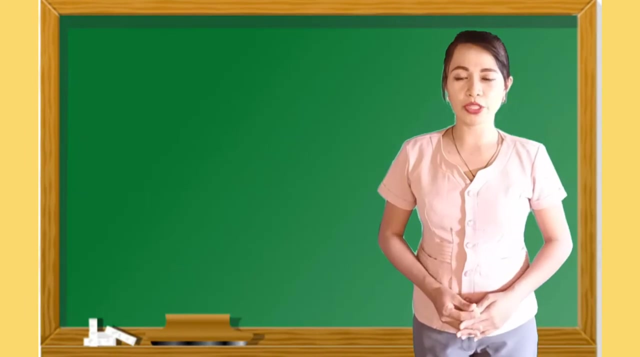 Looking at the illustration, we can say that 1 fourth of 12 is 3.. Therefore, Marcus gave 3 marbles to Arnold. Another way to solve the problem is through computation. There are rules in multiplying fractions, Rule number 1.. 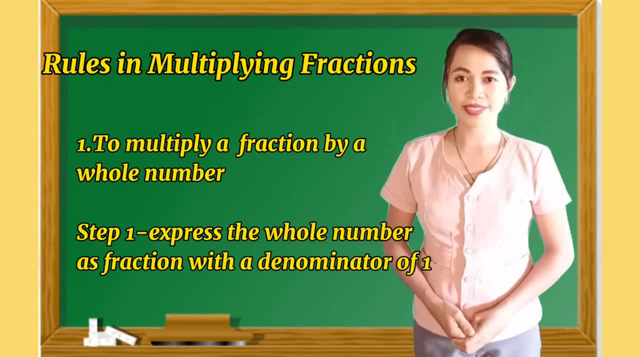 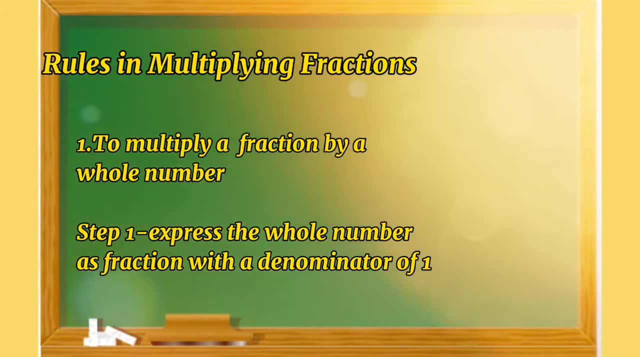 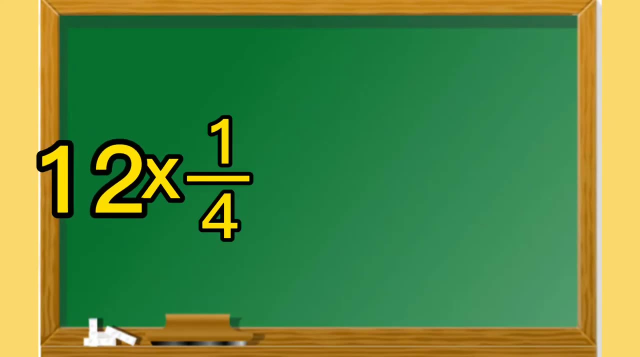 To multiply a fraction by a whole number. Here are the steps to follow. Step number 1. Express the whole number as a fraction with a denominator of 1.. Let's say, for example, from the given problem above, Our whole number here is 12.. 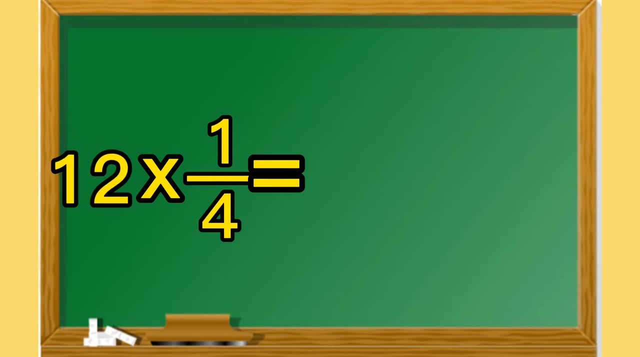 So we just express this as a fraction with a denominator of 1.. So why 1?? That is because whenever we divide 12 by 1, the result is 12.. So always remember, if the given is whole number, just put 1 as their denominator. 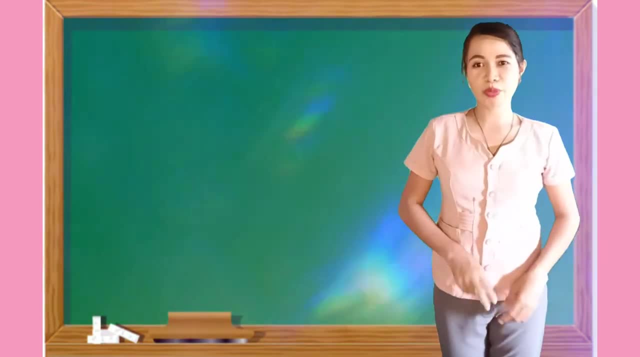 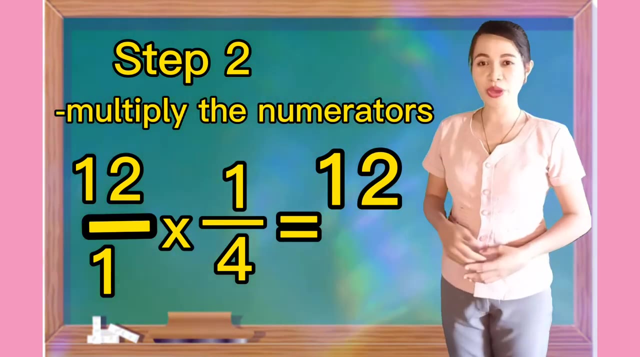 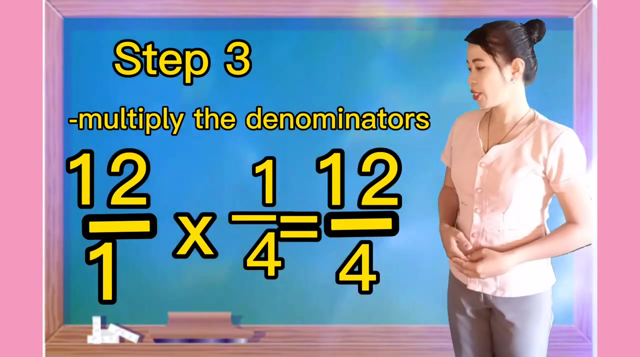 Step number 2. Multiply numerators. Our numerators here is 1 times 12.. The answer is 12.. Next step, number 3. Multiply denominators. Our denominators is 4 and 1.. The answer is 4.. 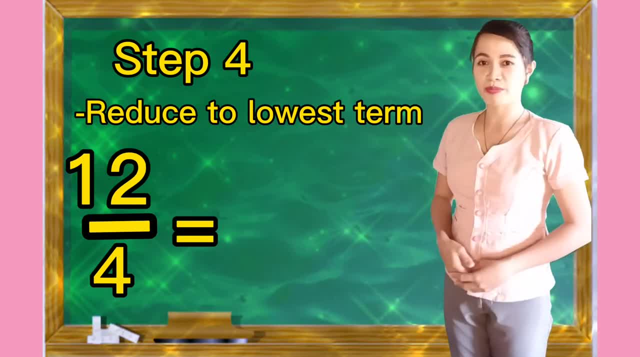 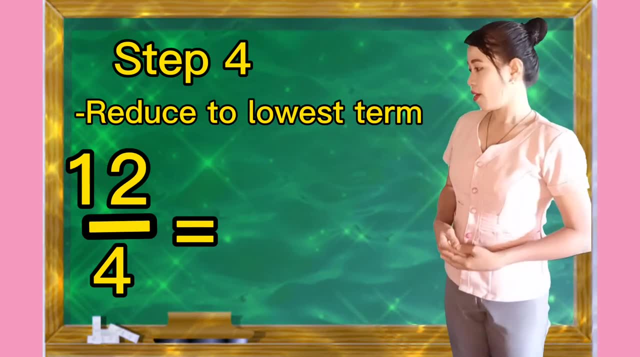 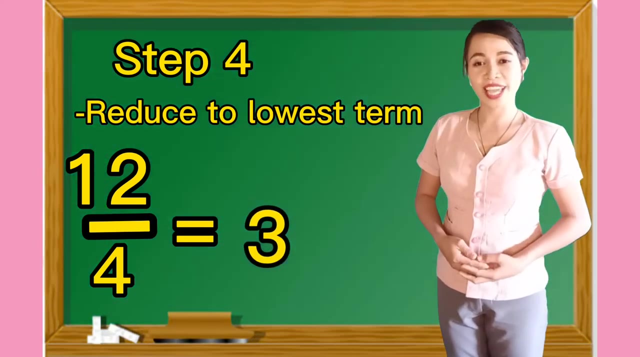 And the last step is reduce to lowest term. Since 12 over 4 is an improper fraction, we need to divide that 1.. So 12 divided by 4 is equal to 3.. So our answer now is the same. So, therefore, Marcus gave 3 marbles to Arnold. 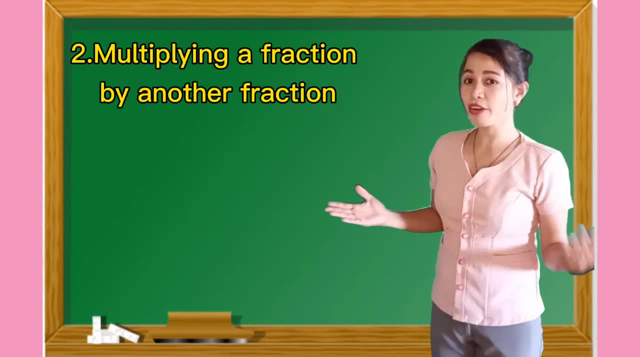 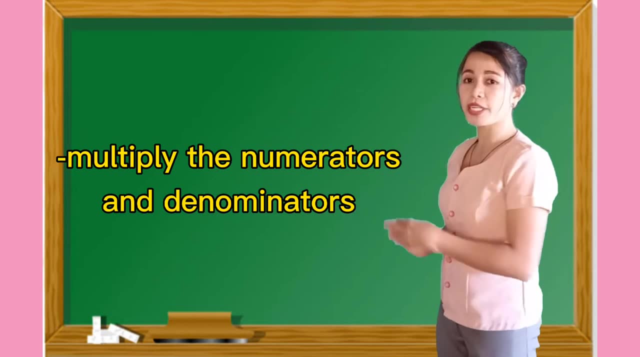 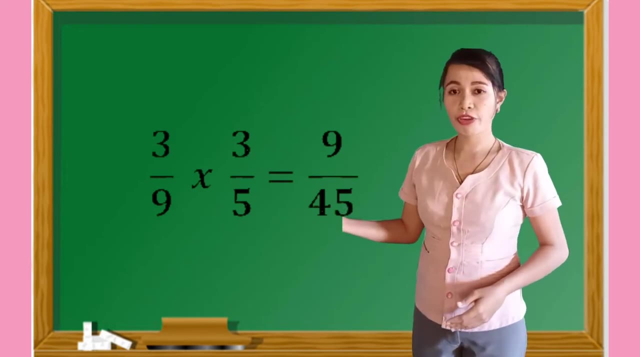 Next, multiplying fractions with another fractions. Since they are both in fraction form, we have to multiply their numerators and denominators directly. For example, 3 over 9 times 3. fifth, So we have to multiply first the numerators, which is 9.. 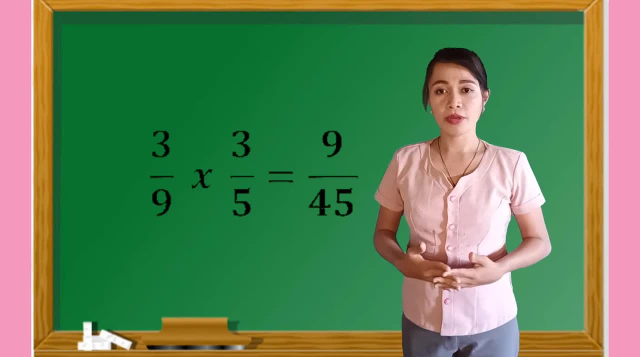 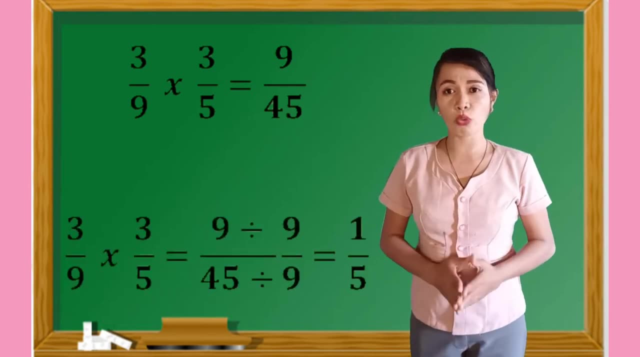 And their denominator goes to 45. So the answer now here is 9 over 45. So 9 and 45 is not yet in the lowest term. We have to find their common factors that can be divisible by 9 and 45.. 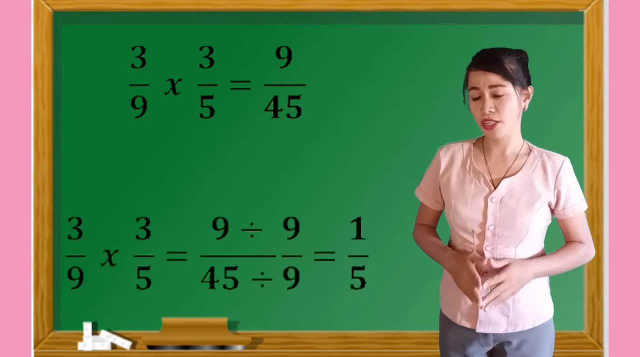 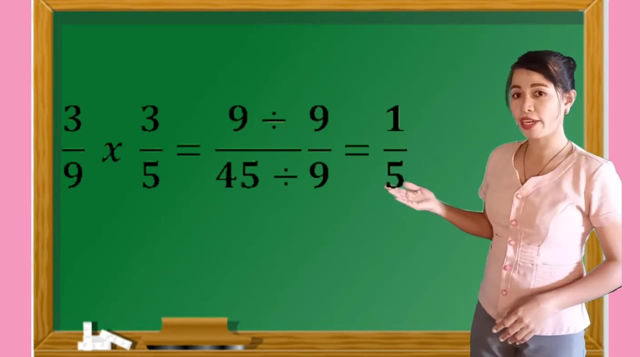 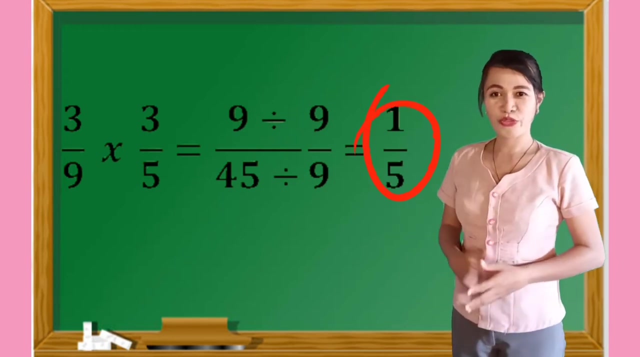 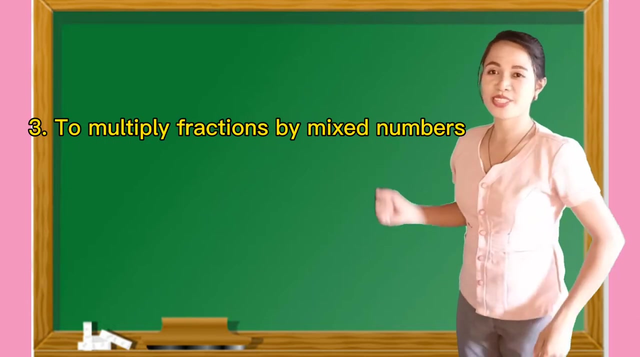 Greatest common factor is 9.. So this 9 divided by 9 is equal to 1.. And this 45 divided by 9 is equal to 5.. So the answer now here is 1. fifth Next, Multiplying fractions by mixed number. 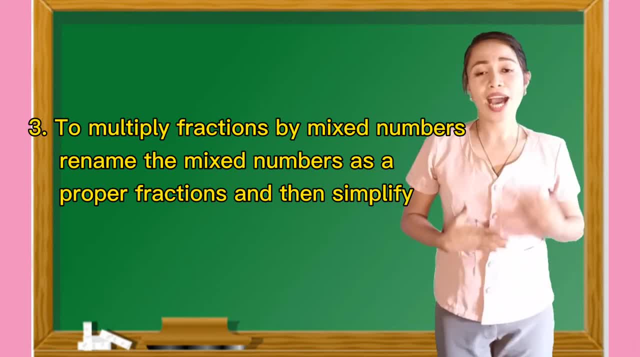 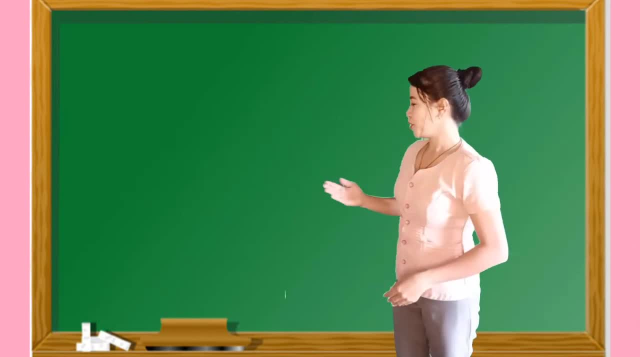 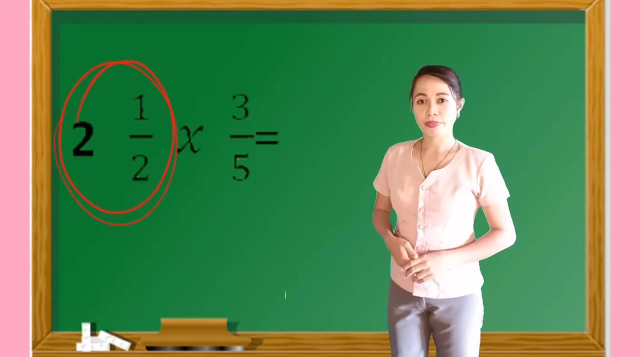 In multiplying fraction by mixed numbers, we have to rename the mixed numbers as a proper fraction and then simplify. For example, 2 and 1 half times 3. fifth, Our mixed number here is 2 and 1 half. In order to rename this 1 into proper fraction, 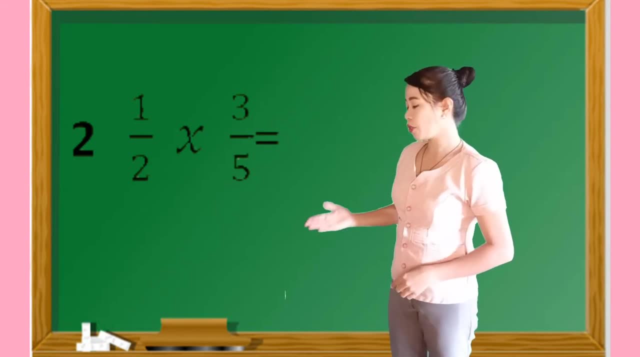 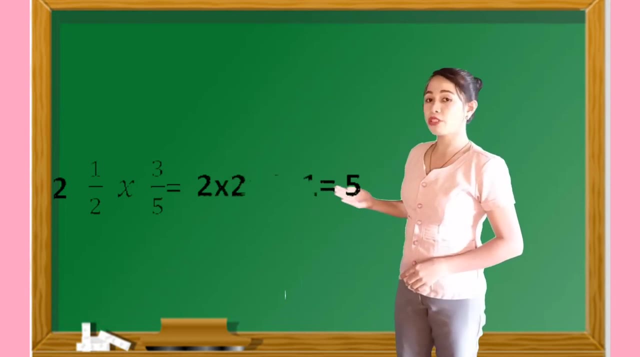 we have to multiply the denominator and the whole number. So our whole number here is 2 and our denominator here is 2.. So 2 times 2 is equal to 4.. After that we have to add their numerator. So the numerator here is 1.. 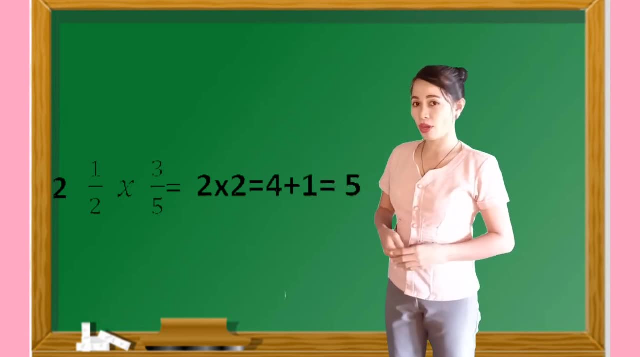 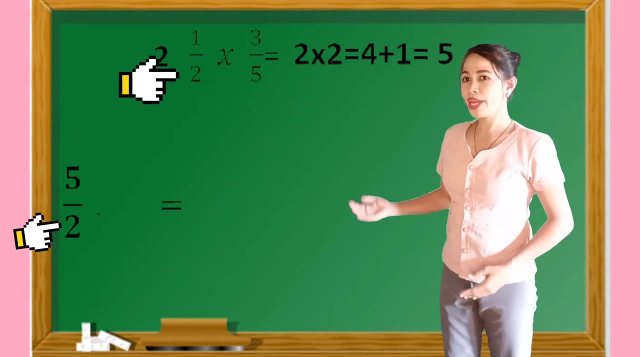 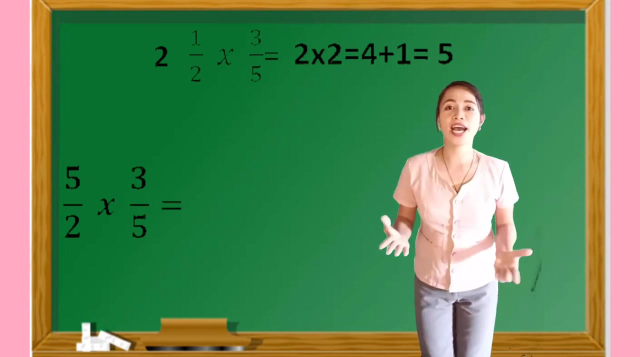 So 4 plus 1 is equal to 5.. And copy the denominator, which is 2.. So 2 and 1 half is equal to 5 over 2.. After that we will going to multiply their numerators and their denominators. 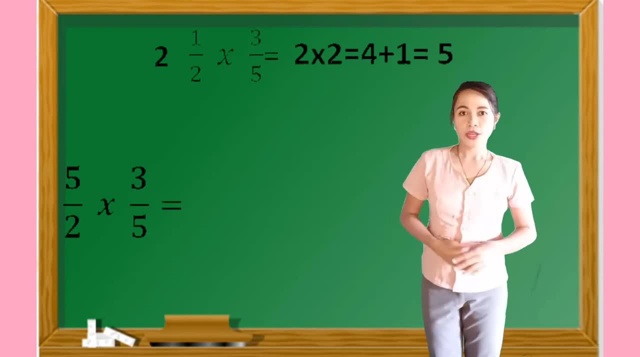 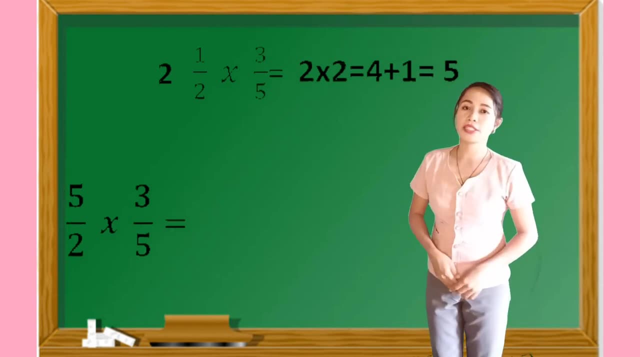 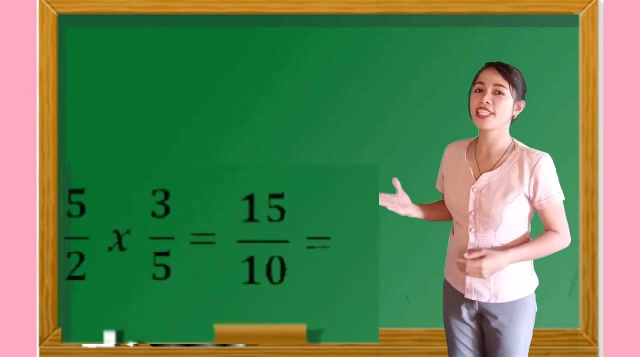 So we have 5 over 2 times 3. fifth, So their numerator is: 5 times 3 is equal to 15.. And their denominator is 2 and 5 is equal to 10.. Okay, 15 over 10 is an improper fraction. 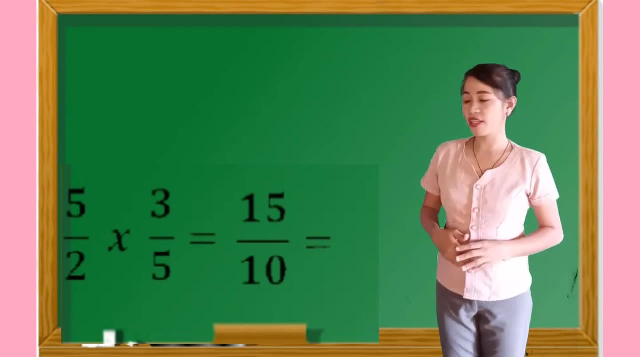 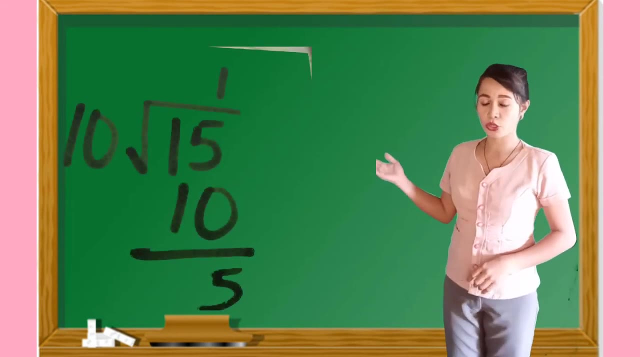 So we have to divide that 1.. So 15 will be the dividend And then 10 is the divisor. So we have: 15 divided by 10 is equal to 1.. And then 1 times 10 is equal to 10, remainder 5.. 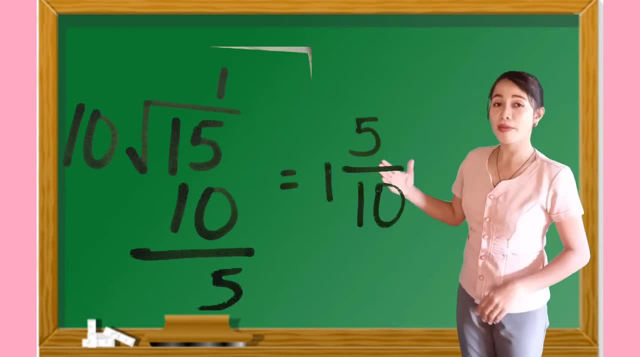 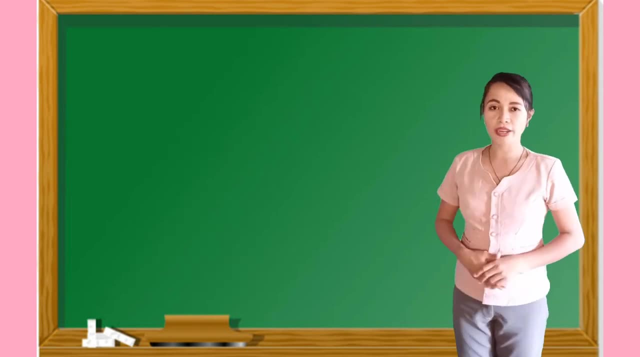 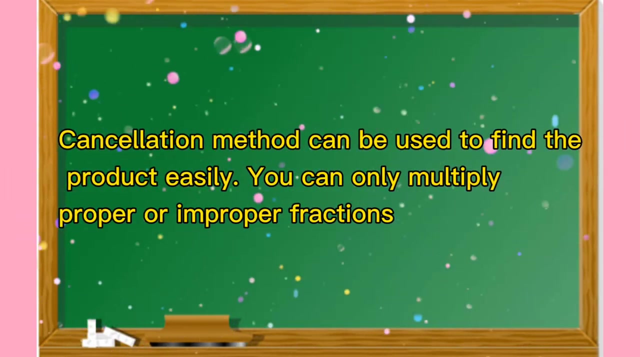 The answer 1 is the whole number, The remainder, 5, is the numerator And the divisor, 10, is the denominator. So the answer now here is 1 and 5, 10.. Another way to find the product easily is by using the conciliation method. 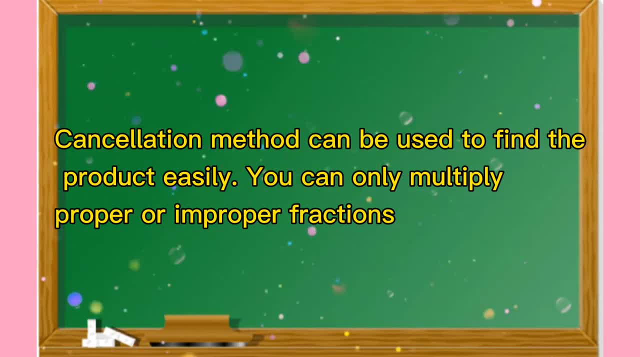 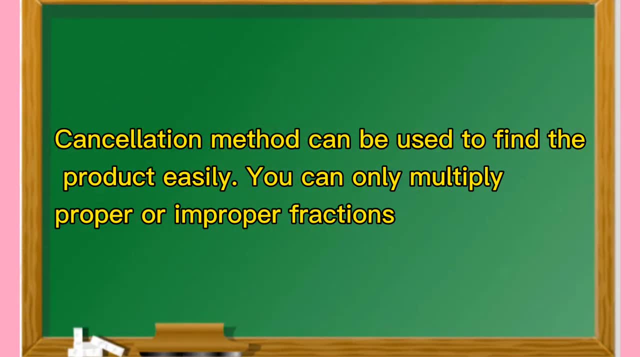 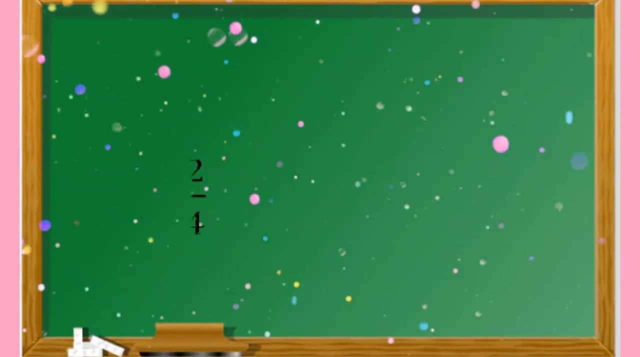 You can only multiply proper or improper fractions, But don't forget to simplify or reduce your answers in its lowest term By using this method. let's try multiplying mixed numbers by a fraction using conciliation method. For example, 6 and 2. third times 2. fourth. 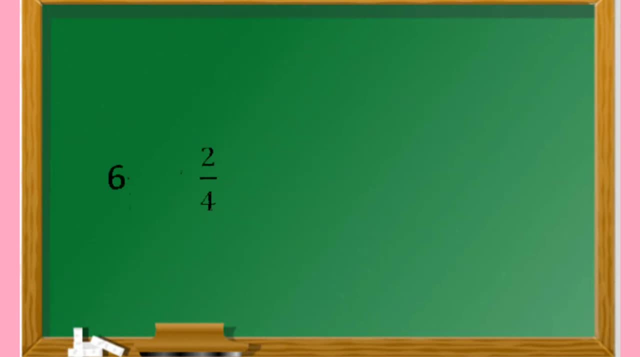 The first thing to do is to rename the mixed numbers as proper fractions, So our mixed numbers are now called mixed numbers. The number here is 6 and 2 third. So we are going to multiply the whole number with the denominator 3.. 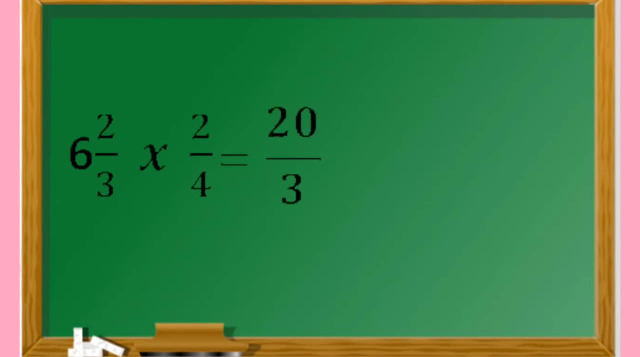 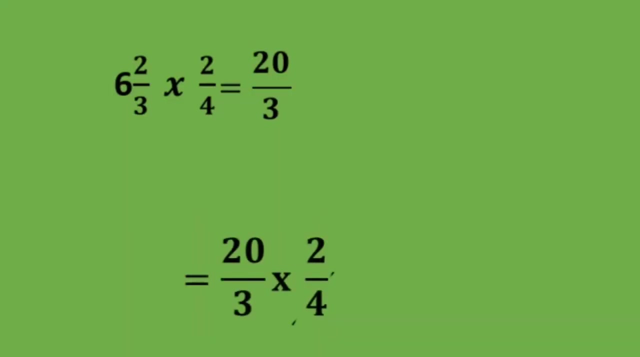 So we have: 6 times 3 is equal to 18. And add the numerator 2.. So a total of 20.. And copy the denominator of 3. Then our proper fraction now is 20 over 3.. After that you have to look for a pair of numerator or denominator to conceal or reduce. 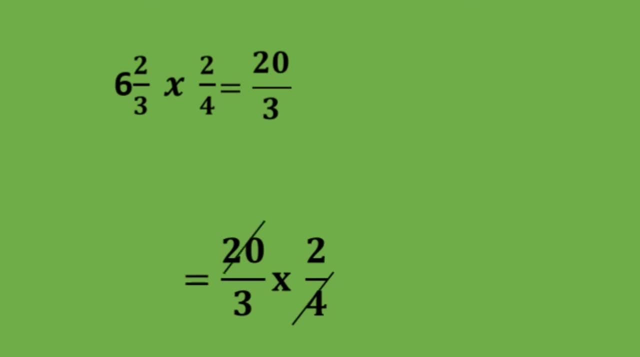 Then multiply, We have 20. And 4.. Because 20 and 4 has a denominator of 4.. So 20 will be divided by 4, will become 5. And 4 divided by 4 will become 1.. 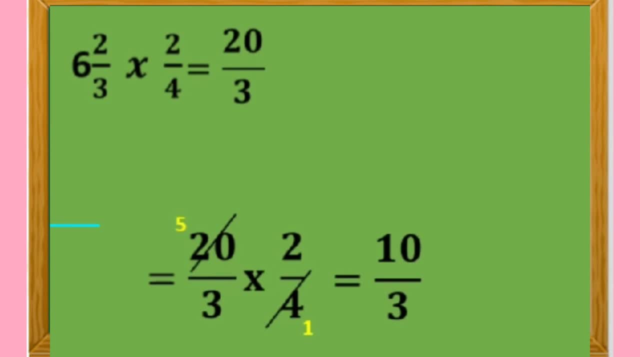 So 5 times 2 will become 10. And 3 times 1 is equal to 3.. So 10 over 3.. Do you think 10 over 3 is in the lowest term? Of course not, Because this is an improper fraction. 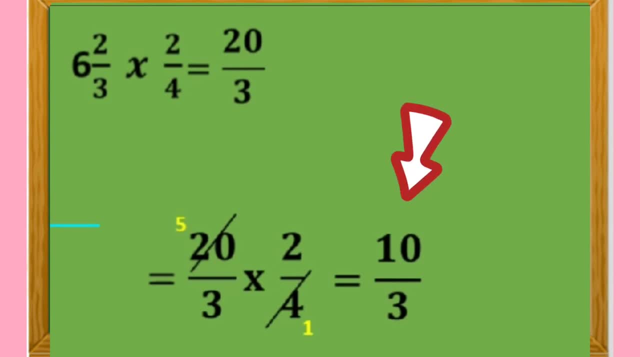 So we have to divide this: 1.. So 10 will be the dividend And then 3 will be the divisor. So 10 divided by 3 is equal to 3.. And then 3 times 3 is equal to 9.. 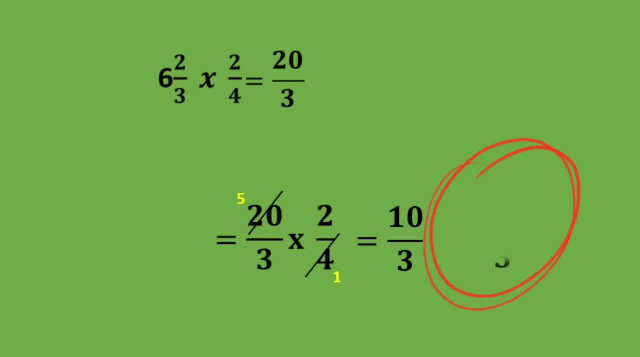 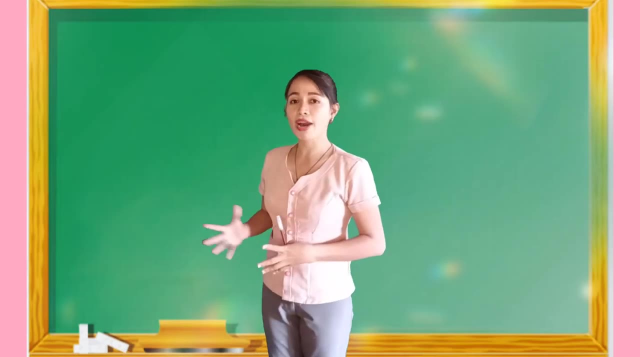 Remainder 1.. So the answer now here is 3 and 1. third, Conciliation is very helpful, Since it simplifies the fractions Before the actual multiplication, Thus making the process a lot easier. It is said that practice makes perfect. 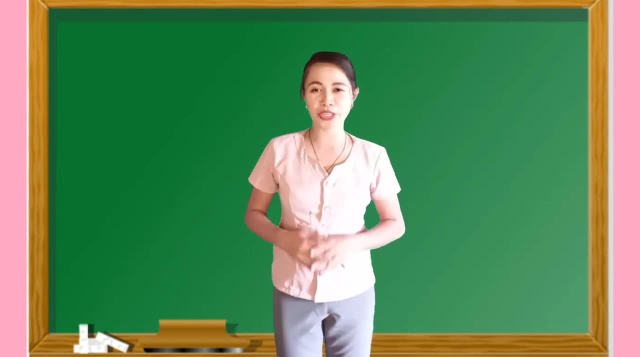 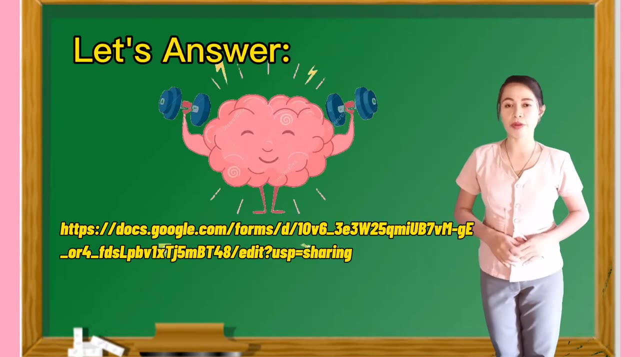 So I want you to be perfect, So I am preparing another set for you to practice on. So let's answer this. Just click the link below for the google form where you can write your answers. I will give you 10 minutes to answer that one. 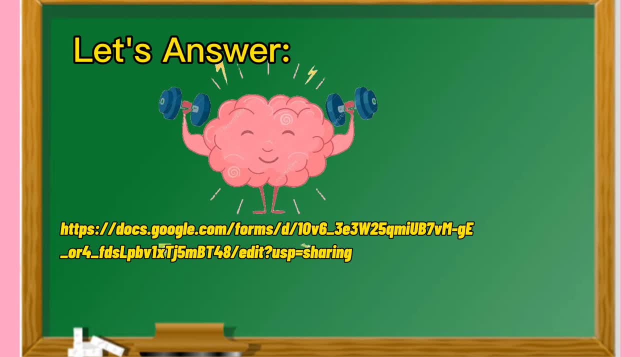 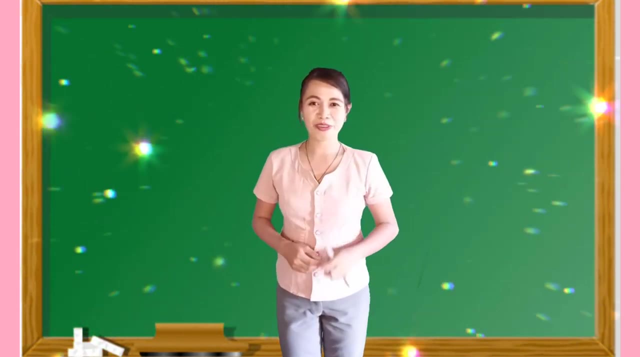 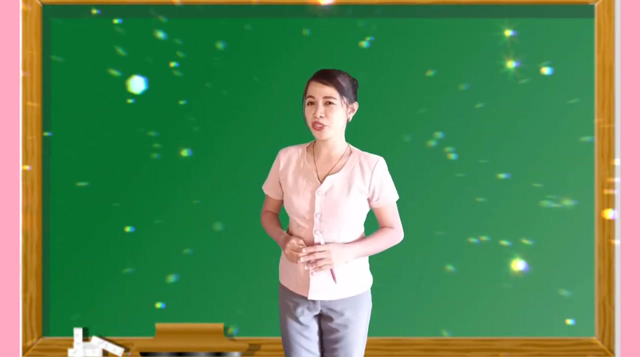 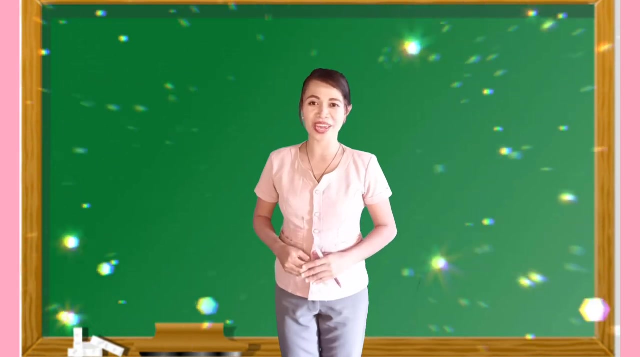 Now let's try. Done answering Very well. Now, how much did you get? If your score is high, that means you are exceptional, And if you get a low score, That shows you missed. that shows you missed something along the way. feel free to go back where you find it hard.